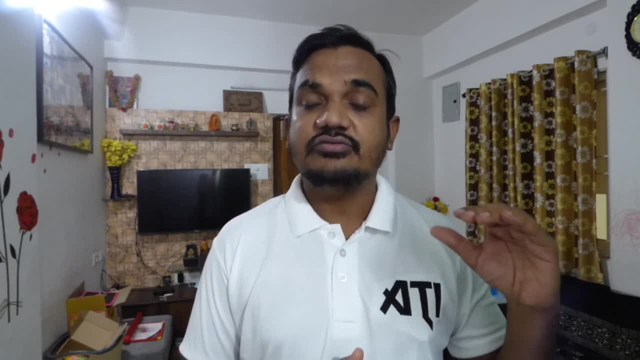 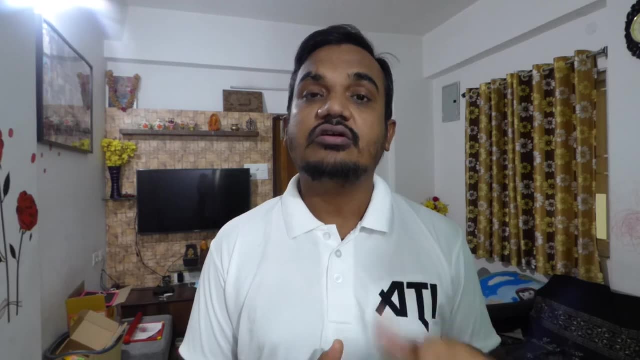 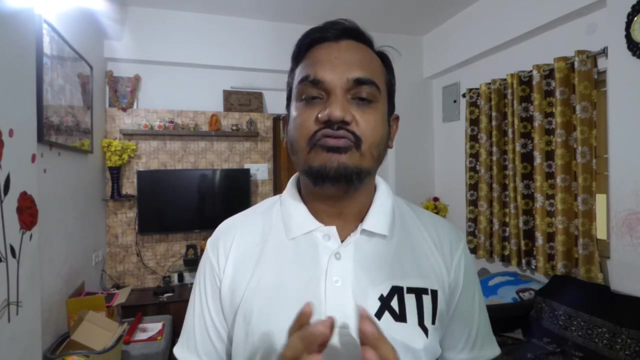 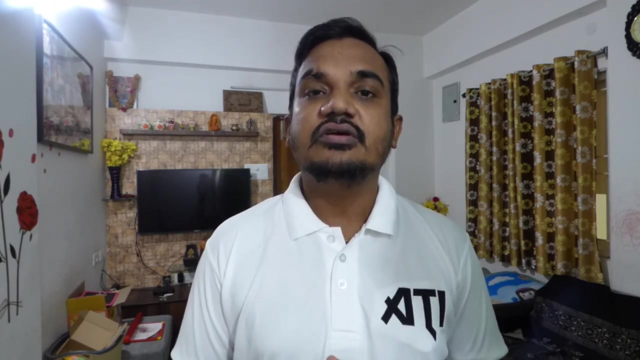 And another thing is until, unless, if our first phase is not done, then we cannot jump to the next phase And also we cannot come back from the next phase to the first phase. So these are the main drawbacks of waterfall model. So to overcome all these drawbacks here we go for iterative model. 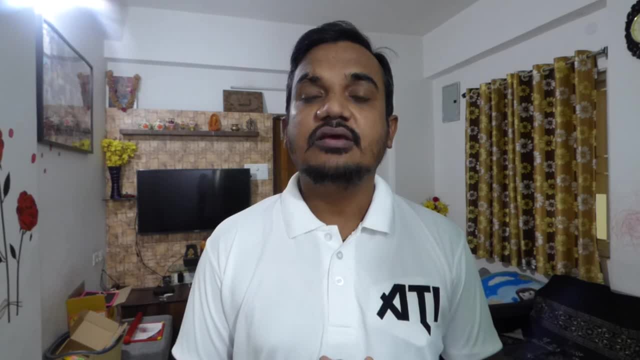 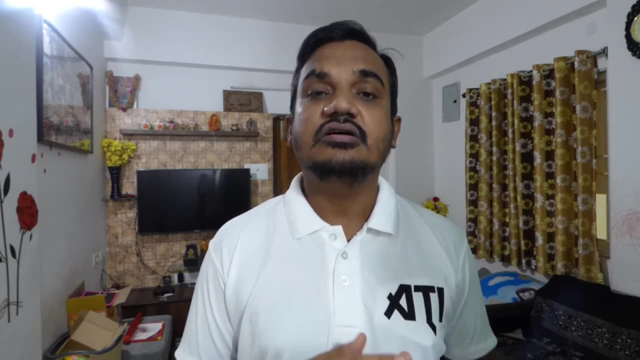 Okay, so what is iterative model? The name says iterative, So it works on the basis of iteration. Iteration is nothing, but when we do something again and again, When we perform some task again and again, it's called iteration. So let me explain. like, what do you mean by iterative model? So take an example. we have some requirements from the customer. Let's say we have X, Y, Z requirements from the customer. 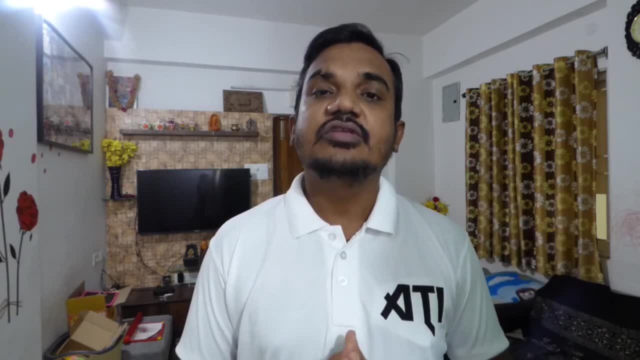 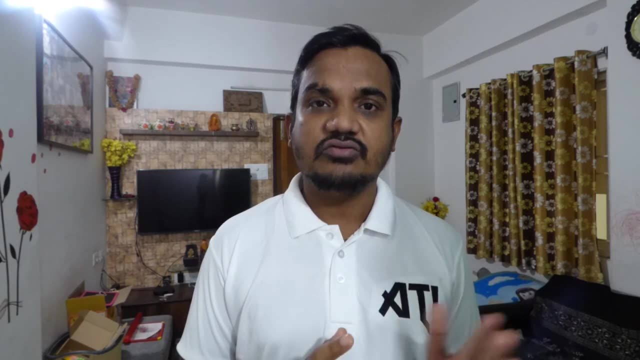 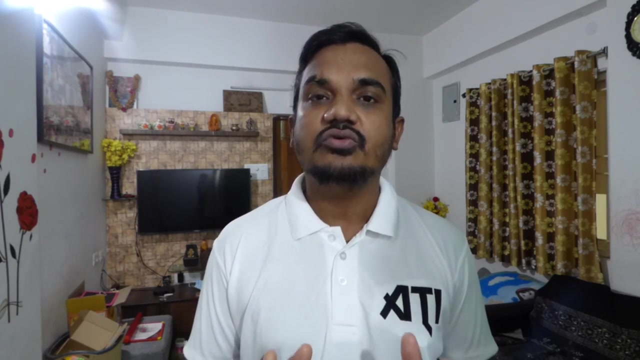 Now, the first is iterative model. So the second step in iterative model is we should prioritize our requirements. So take an example: in this case I'll first go for the requirement X, Okay, and then we'll follow the complete HDLC process, like requirement analysis, design, coding, testing and release and maintenance. 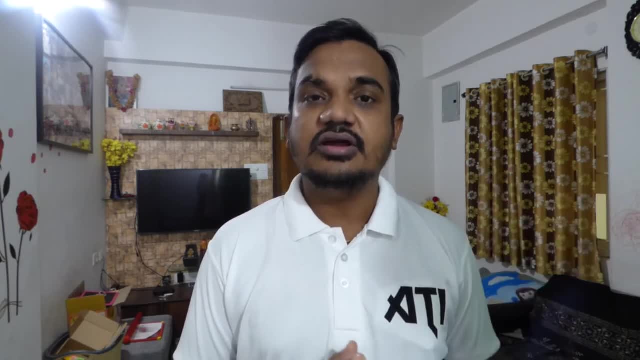 So I'll: I have picked one requirement at a time, like X, And then we follow the waterfall, like: what are the different HDLC phases? we have requirement analysis, design, coding, testing and release and maintenance. So then I have pick one requirement at a time, like X, and then we follow the waterfall, like: what are the 것이 phases? we have requirement analysis, design, coding, testing and release. and maintenance requires. 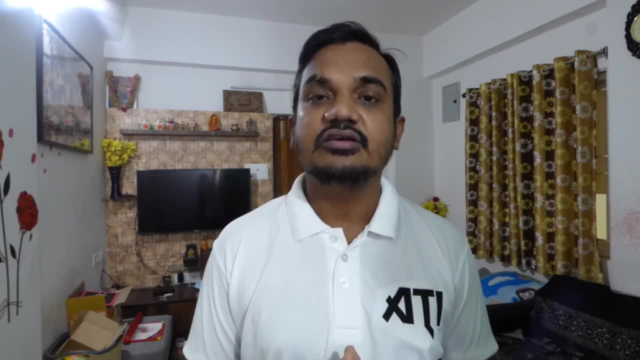 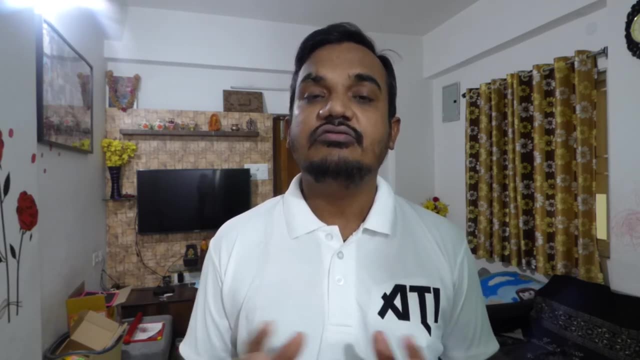 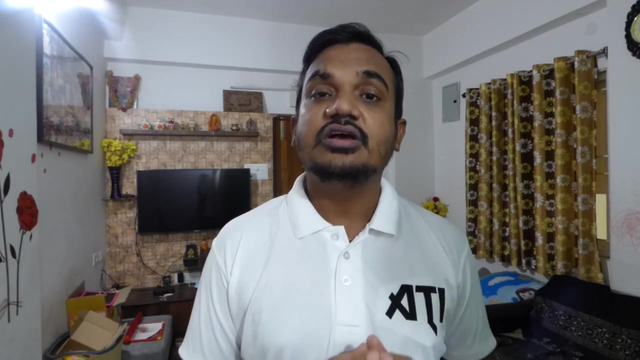 Okay, analysis, design, coding, testing and release and maintenance release: okay. so we'll follow all those steps and we'll deliver the first build of software, working software. so this is first iteration. now, after getting the feedback from the customer, getting the feedback and reviews from the customer will work for the requirement y. now again, we'll perform the same task like requirement. 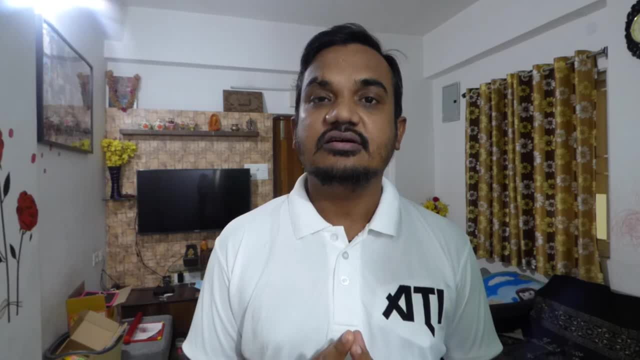 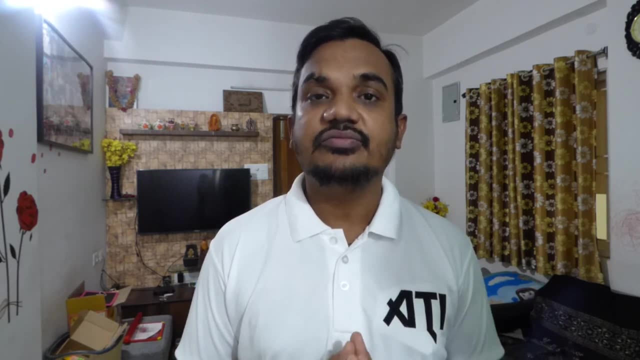 analysis, design, coding, testing and release. so this is iteration two. similarly for uh, the third requirement, that is y, uh, z, x, y, z. so the z. the last one is z. so we'll work for the uh, same pro. we'll follow the same process for requirement z. 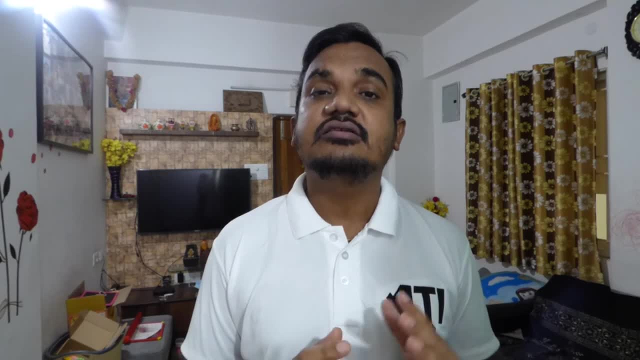 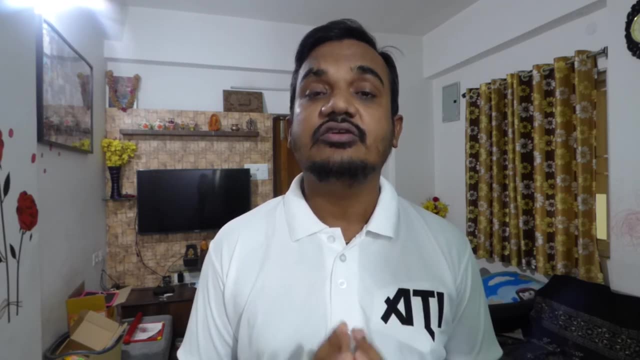 so we'll follow the same procedure again and again till we get gets the final build. so this is how iteration works. okay, this is called the iterative model. so let me take you to my PPT, where we'll discuss, like some, some of the theoretical stuff of 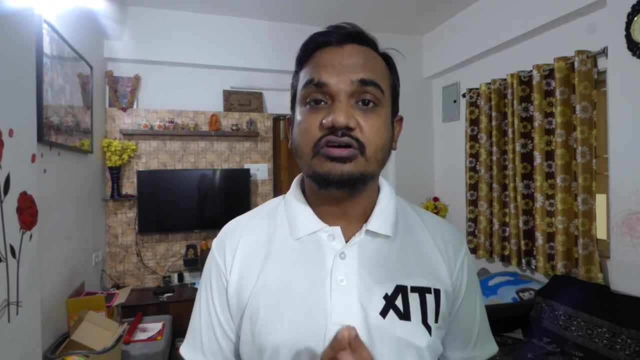 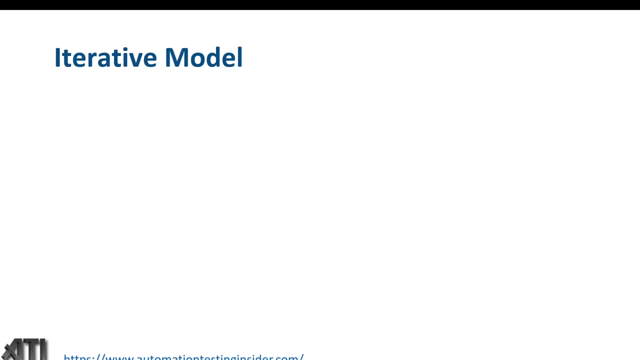 iterative model and also discuss about pros and cons of iterative model, and I will show you. I'll explain you better with the help of diagram there. so let me take you to my PPT. guys, let me just recap what we have discussed at the beginning of this video, some theoretical stuff so you can make a. 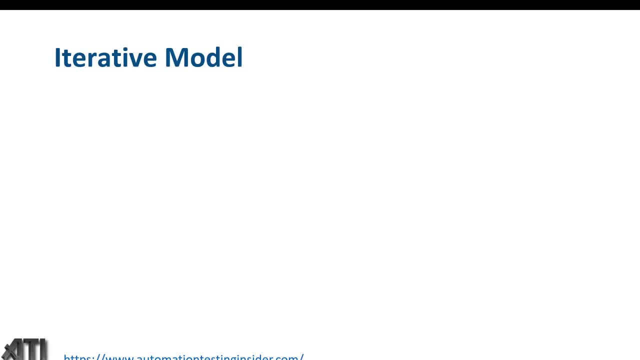 note of it like: what do you mean by iterative model? how it works? so we create rough product or product piece in one iteration, then review it and improve it in the next iteration, and so on until it's finished. so we work on the basis of like it's. it works on the basis of module. 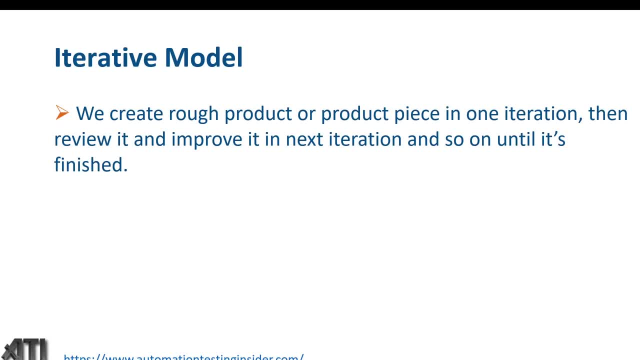 module wise, and then we'll get some reviews from the customer, so we'll work like module 1, module 1, 2, 3 and so on till we get the final build, and in the next slide I'll show you, with the help of example, whatever we have discussed at. 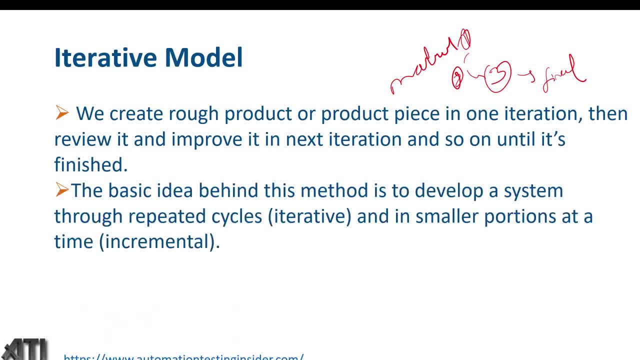 the beginning of this video. so the basic idea behind this method is to overlap, develop a system through repeated cycle, iterative, iterative and it is, and in a smaller portion at a time, incremental. so this is also called incremental model. ok, so this is the combination of iterative plus incremental. why it is called incremental? because it increments the 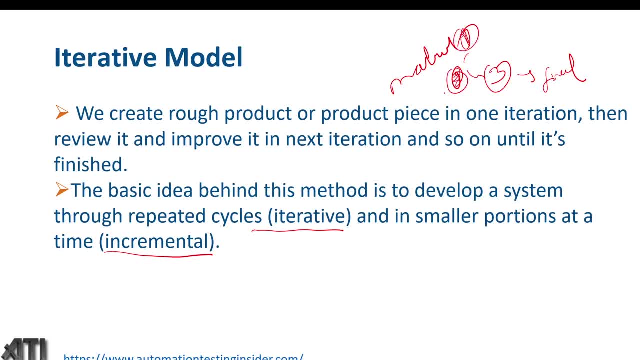 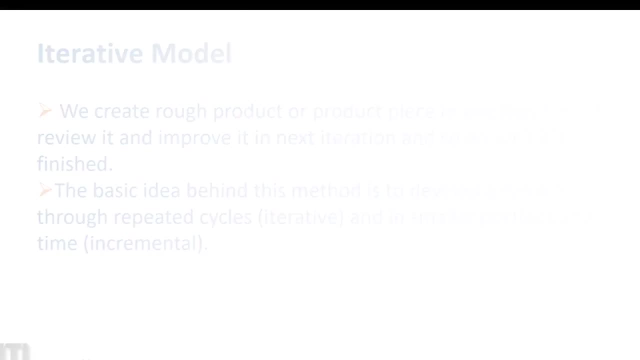 requirements like module 1, module 2, we got some other requirements and then module 3, so we incrementally adding all those requirements, those modules. so that's why it is called incremental module as well. now let me explain the help of an example. so suppose we got some requirements from the customer. take an: 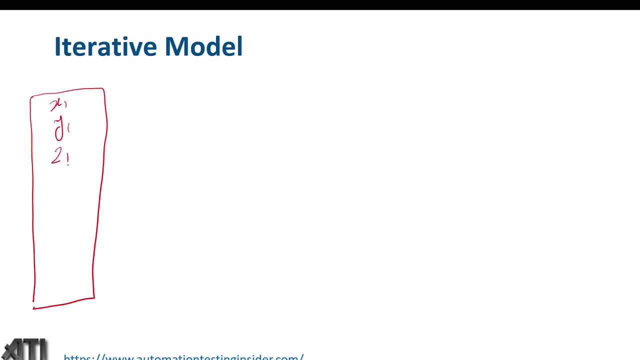 example, this is requirement x1, y1, z1, x2, y2, z2 and x3, y3, z3. so these are the requirements we got from the customer environment, from the customer. now we'll follow the SDLC process, the complete SDLC process, to build the software in. 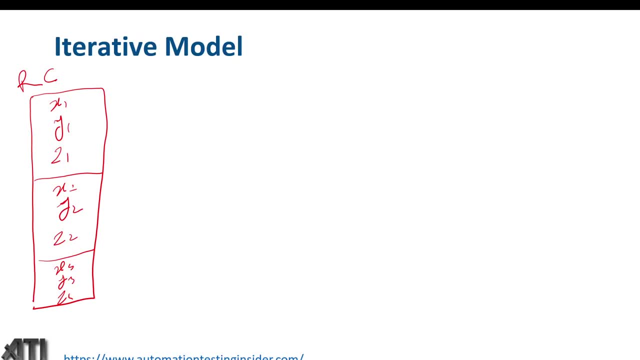 the previous slide, we have seen like we have to deliver. the first working is of software will follow the complete lifecycle like requirement analysis, then design, design, then coding, just testing, then release and maintenance. at last we we get the feedback with back and reviews from the customer for this build. so this is 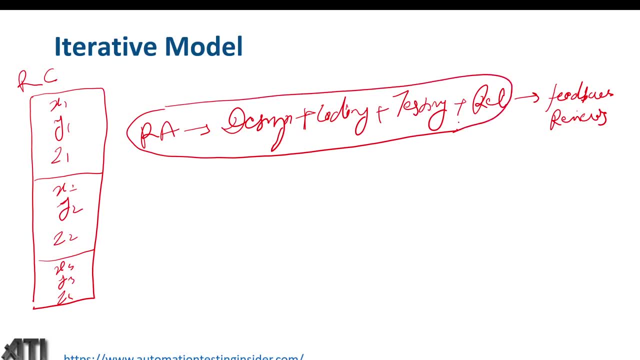 complete one process, guys, and this is called build one. do not worry about the build and release. I'll create a separate video. what do you mean by build and release? so we followed the first module will, and this is considered. consider this is module one. okay, consider this is module module one. 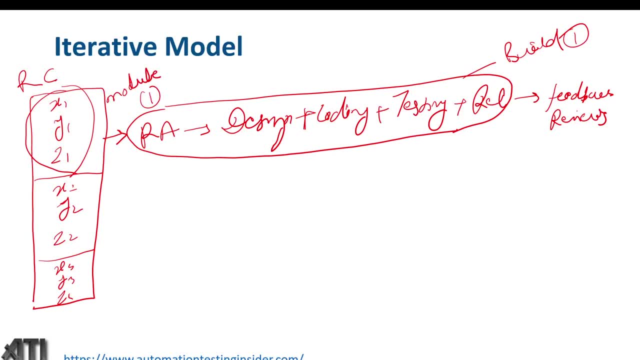 this set of requirements under module one. now we followed the complete step so this is called iteration one. iteration one: now we got some feedback from the customer and reviews and will work based on those reviews and feedback will work on module two. we'll keep. we add those feedback and reviews in module two. okay, suppose they. 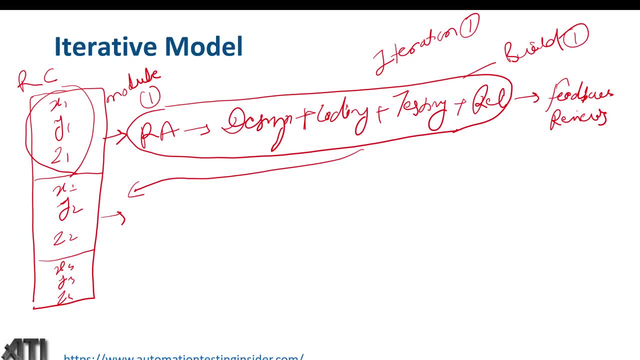 want to make some changes in module one, so we'll make the correction and will integrate with module two. now we develop a module two along with module one. now we'll follow the same procedure again and again: requirement analysis, design, coding, testing and release. so this is iteration. 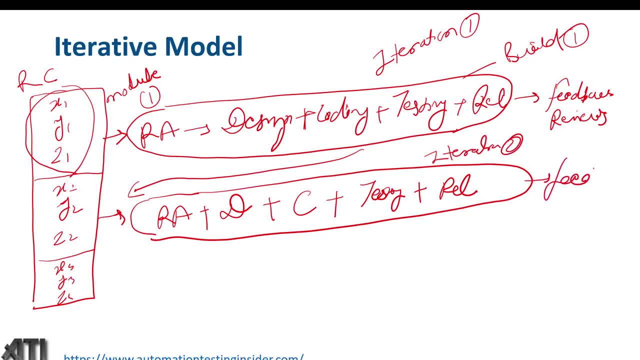 two. now again we'll get feedback from the customer reviews from the customer. okay, now we'll develop module three. so we'll keep adding module one, two, three and so on till we get our final build, final product. so this is how it works, the iterative model. it is called incremental why? because we keep 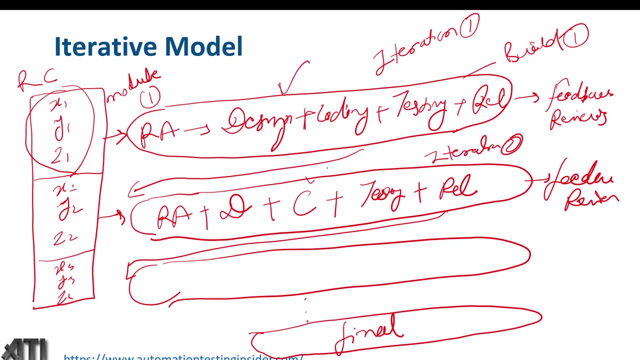 adding module 1, module 1 plus module 2 plus module 3, and so on. that's way it is incremental and iterative is called incremental. it is why it is called as it is, because we know that moduleóc, because this is. we follow the same procedure again, again and again. okay, so this is one. 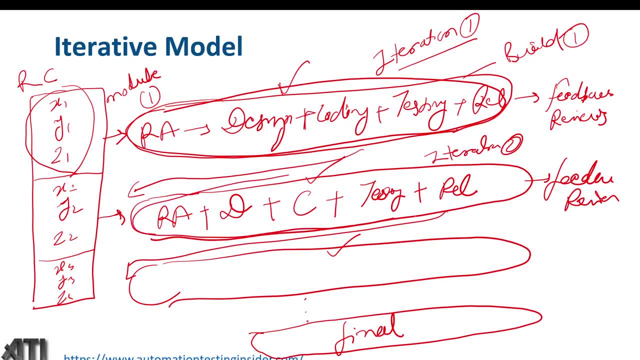 hdlc process, iteration one. this is again we followed the hdlc phase, iteration two, and this is iteration t, so this is about iterative model. and another thing is like module two can start parallelly as well, because we have already working on module one, now we can start. 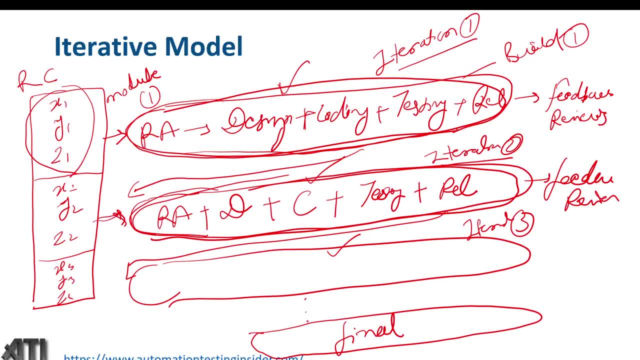 start module 2 as well at the same time. maybe after it is it reached over here coding phase, then we can start parallelly module 2 as well from requirement analysis, so it can run parallelly as well and it works for the project which which has multiple modules, like in this case. 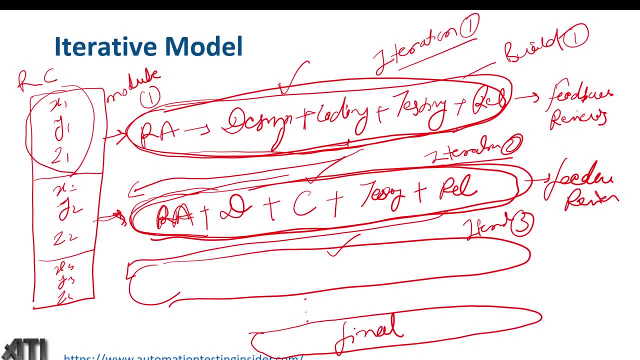 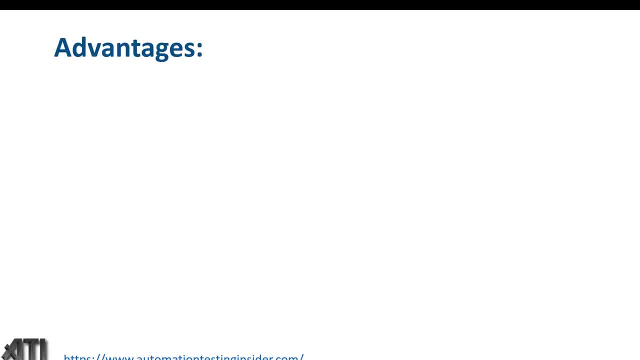 we have. we have divided into three different modules. so this is how it works, guys: iterative model. now let's talk about some advantages and disadvantages of iterative model. so testing and debugging during smaller iteration is easy. we have divided into different modules, so debugging is easy. in this case it is easily acceptable to ever changing needs of the project. 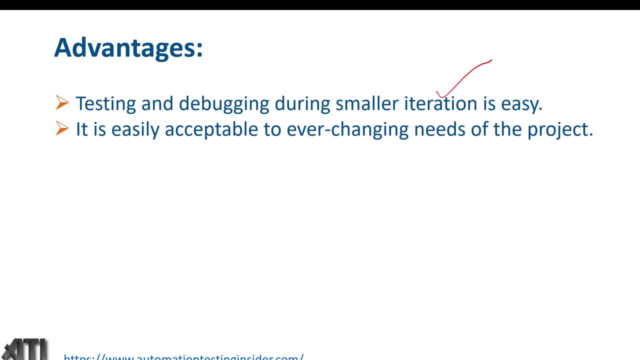 so in this is the biggest drawback in in waterfall model, like we cannot change the requirements, we cannot come back and change the requirement, but here we can accept the requirements. limited time is spent on documentation and extra time on designing. so this is an important point. so we have we spent less time on documentation and extra time on designing. risk are identified. 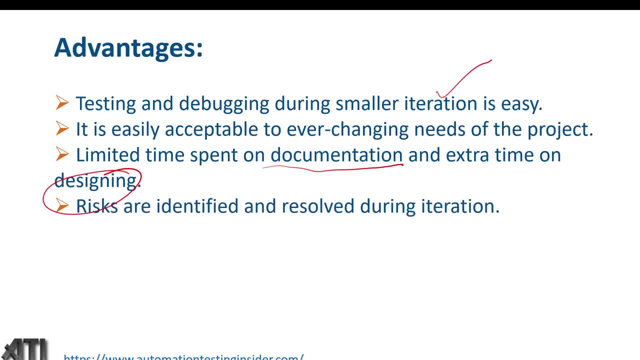 and resolved during iteration. so whatever risk we'll get, we'll talk about risk in the next model. more about some more points about that risk. I'll create a separate video on risk because it's because we have a complete tutorial on risk as well, because that is separate part. so risk are identified and resolved during each. 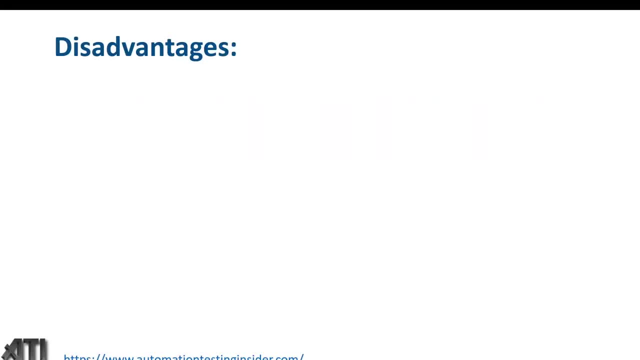 iteration. so what are the different disadvantages of spiral model? so it is not suitable for smaller projects, since we have divided into different modules and we work on the basis of like SDLC and we followed module wise concept. so if cost will be increased if we follow this for smaller projects, okay, so maybe. 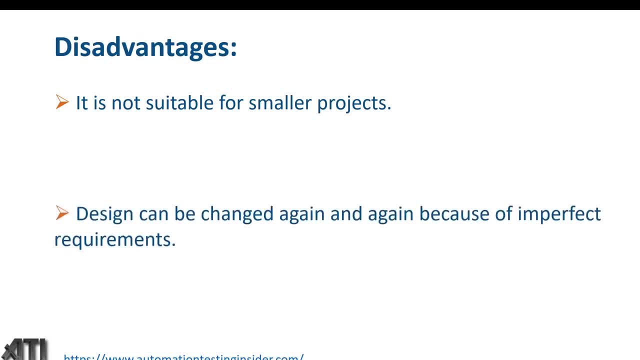 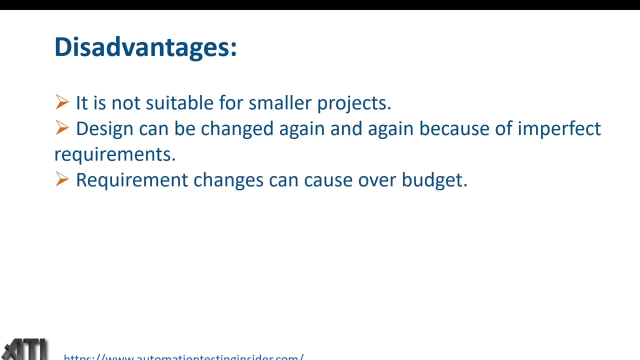 it will not be equal for small projects. design can be changed again and again because of imperfect requirements. so if you don't get the correct requirements then design can be changed again and again. so this will cost. this will double the budget of the project. requirement changes can cause over budget are the same thing and then 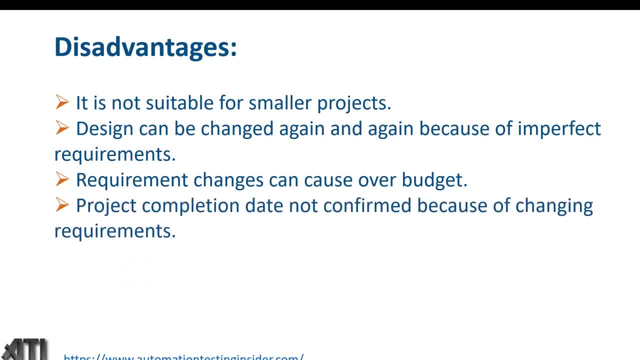 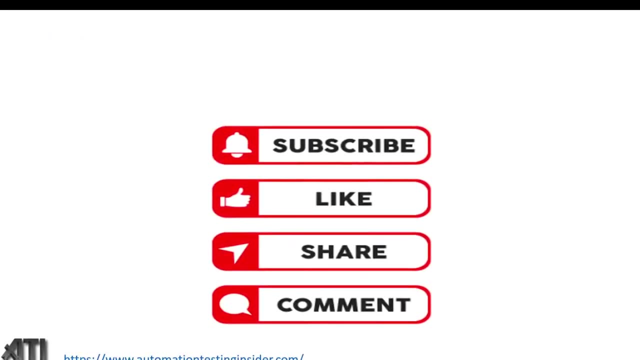 project completion date not confirmed because of changing requirements. yeah, completion date is not confirmed because of the changing requirements. so these are the drawbacks of spiral model, sorry, iterative model. so in the next video, guys, I'm gonna talk about viral model. so thank you, guys, thanks, thank you so much, and please like, share and comment if you have any. 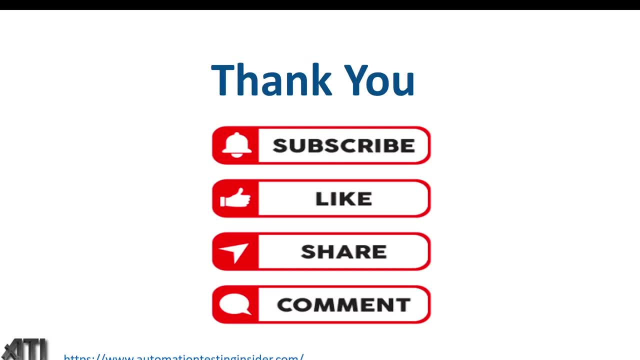 questions and subscribe this channel and click the bell icon to get the notification for upcoming videos. thank you so much. have a nice day, bye, bye.